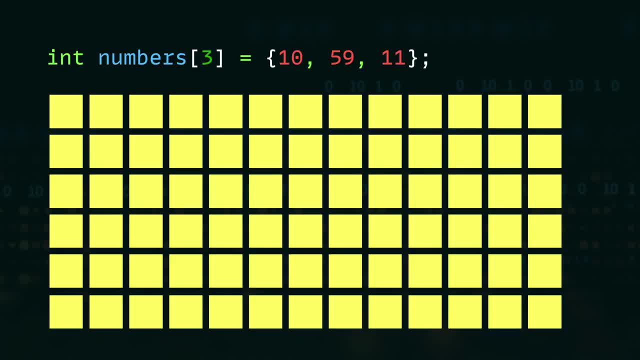 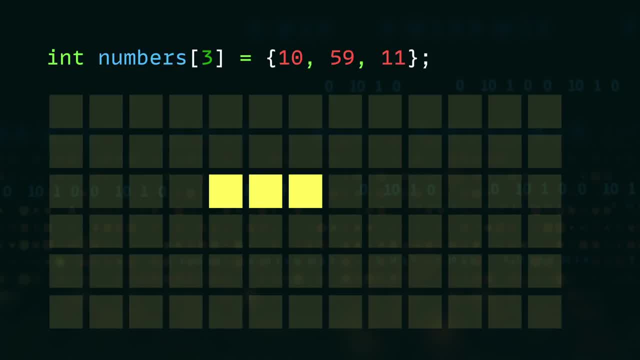 Let's say that we have this array of three integers which we have to represent in the memory. now, what our program is going to do is it is going to allocate three slots in the memory and then it is going to populate the values in those slots. Now, since the computer memory is 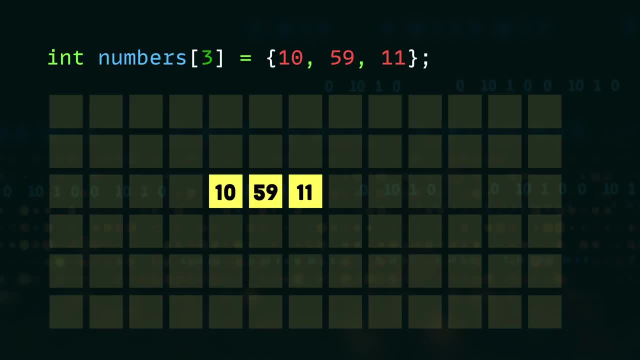 not only specific to us and it is available for the other programs as well. computer is going to keep using these memory slots and keep allocating the memory slots for the other things. Now, later on, let's say that we try to add a fourth element to the array, Since our program allocated only 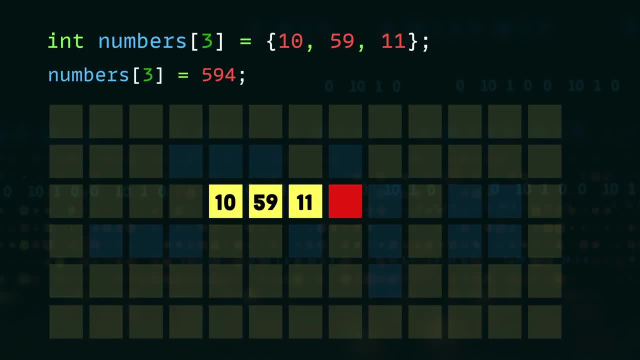 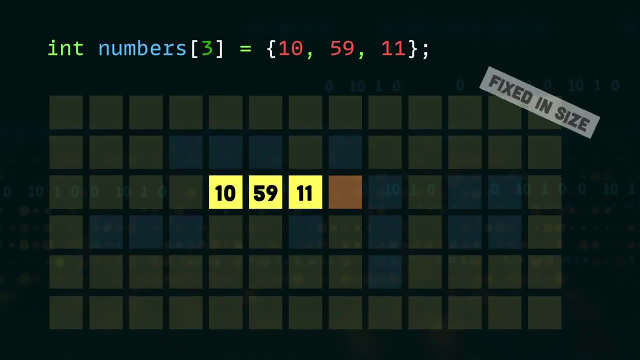 three slots in the array. let's say that we have this array of three integers which we have to slots for the array. the fourth slot may or may not be available, and so the program is not going to allow us to populate the fourth value in the array, and that is the reason why we have the arrays. 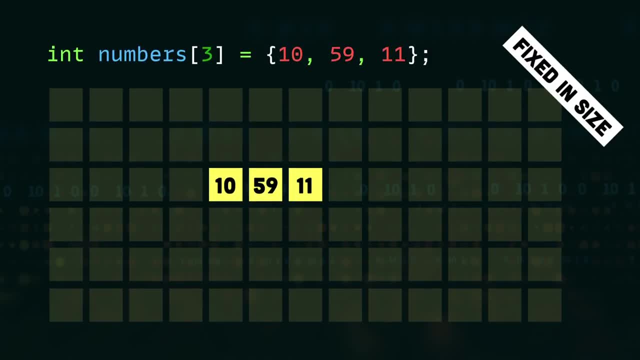 which are fixed in size. so we have to define the size of the array before we start using it, so that the computer can reserve the consecutive memory blocks for the array to be used. now you might be wondering what is stopping us from allocating a really large number for our array so that whenever 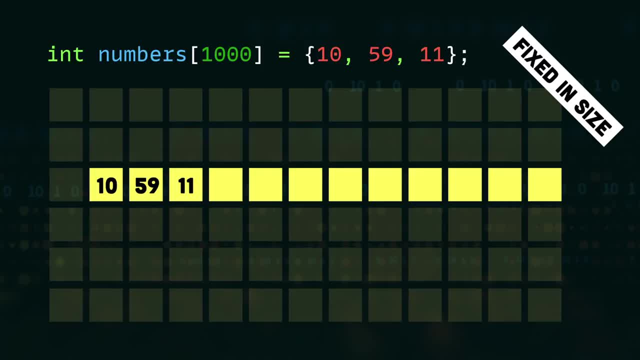 we need new numbers, we can simply push them into the array. the reason why you can't do that is because, in doing so, you'll be keeping all those memory slots for yourself, even if you don't need them, and you won't be letting the other programs which might need those memory slots from using. 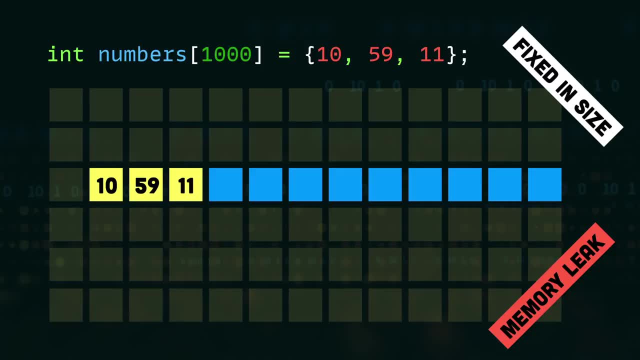 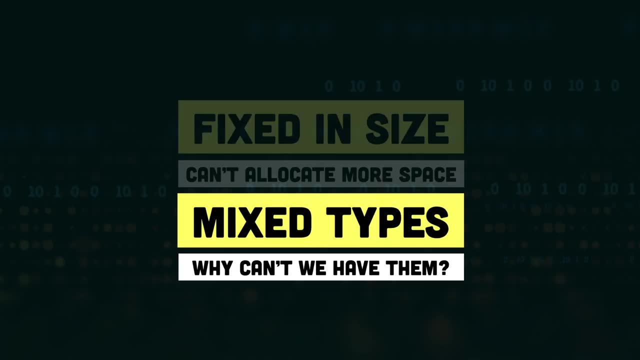 those memory slots and this will cause the memory leak. all right, so next we have the case for the mixed types. why can't we have the areas with the mixed data types? before we talk about that, let's look at some of the example data types. let's say that we have the case for the mixed data types. 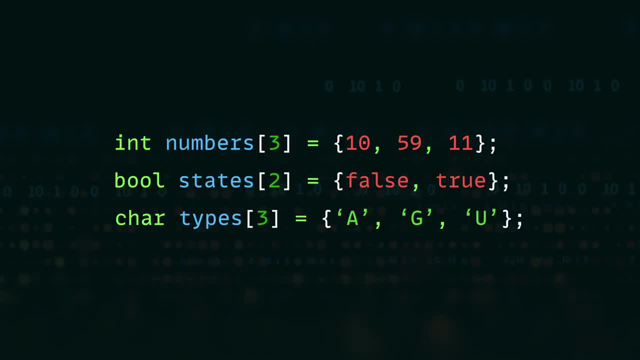 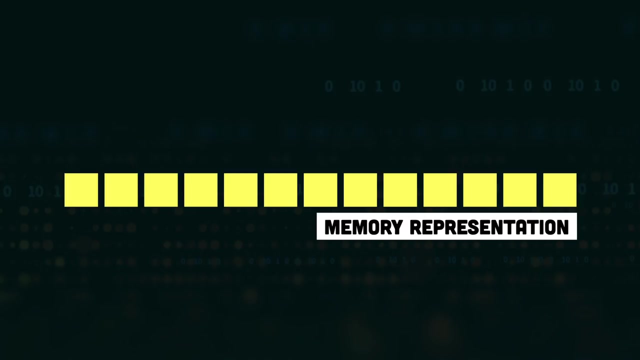 we have these three different arrays: an array of integers, an array of booleans, an array of characters. now, the size of an integer is 2 bytes each. a boolean value takes 1 byte in the memory and a character also takes a single byte in the memory. let's say that we have this memory. 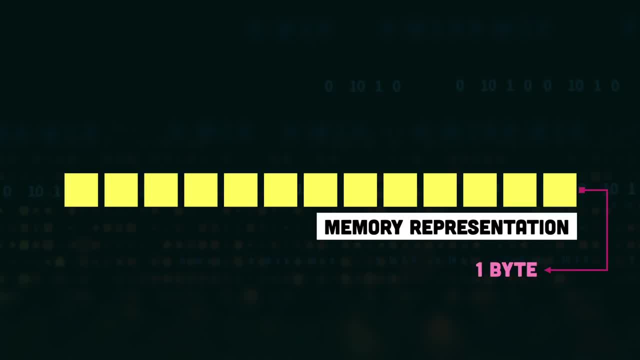 representation where each block represents 1 byte in the memory. let's say that we have this array of integers that we need to represent in the memory. we know that each integer takes 2 bytes in the memory. So the first number in the array, that is 4, it is going to take two blocks or two bytes. 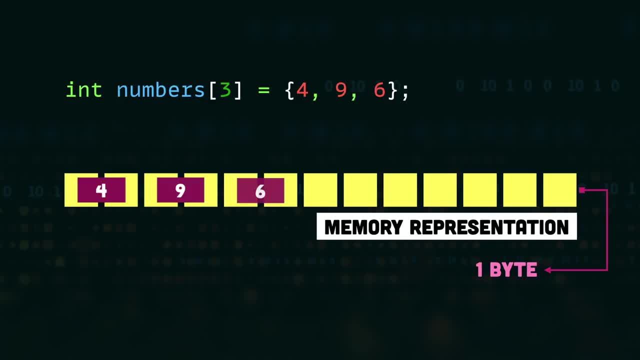 9 is going to take another two blocks and 6 is going to take the last two blocks. Now, when it is time to access these array elements from the memory, since our program knows that the array is an array of integers, so it knows that it has to read the first two bytes and it will get the first number of the. 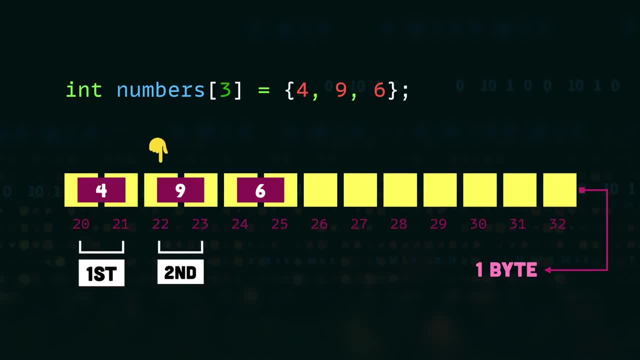 array. Skip two bytes and read the next two bytes and it will get the second number. Skip four bytes and read the next two bytes and it will get the third number, and so on. Now imagine if we had an array with the values of the mixed types. So we have an integer which will take two bytes. 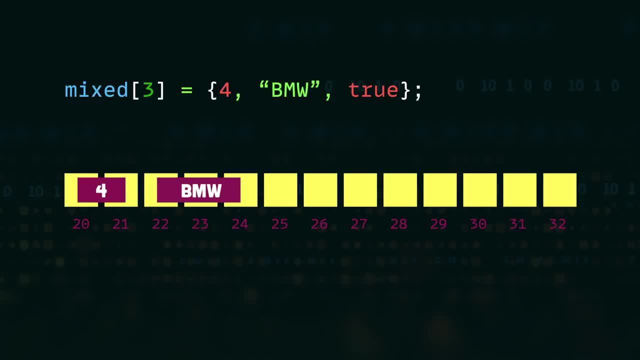 a string of three characters, which will take three bytes, and a boolean which will take one byte. Now, when it is time to read these values from the memory, since it is an array of mixed values, our program won't know how many bytes should it read to get the first, second or third value. 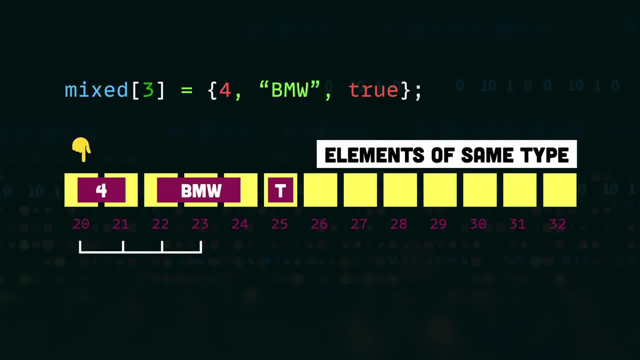 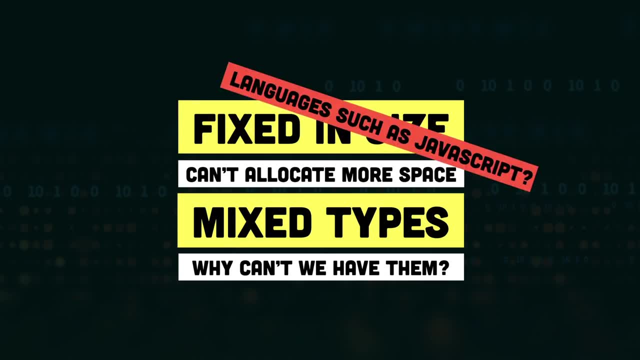 And that is the reason why all the items of an array have to have the same type. Alright, so now you might be wondering: why don't we have these limitations in the languages such as JavaScript, PHP or Ruby? How can we have the dynamically sized arrays and also they support? 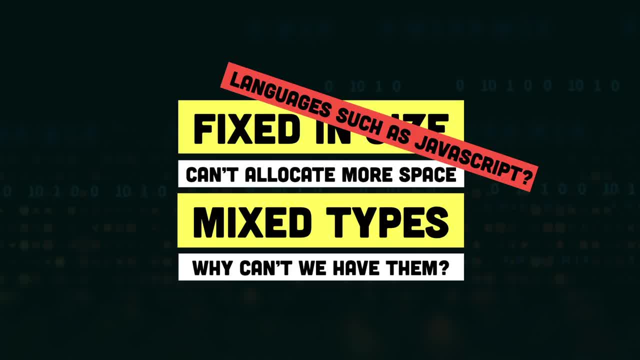 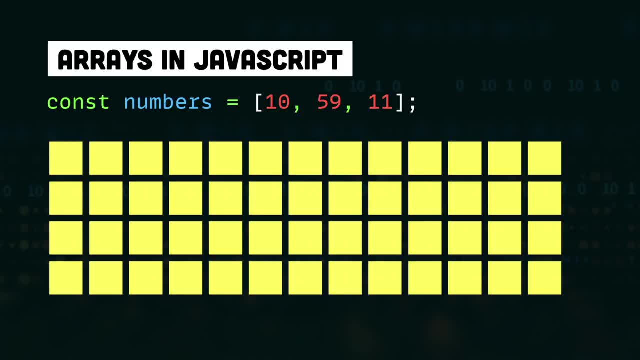 the values with the mixed types. And the answer to that is because there is a lot going on behind the scenes to make it work. Let's say that we have an array of numbers in JavaScript. It's going to allocate three blocks and populate the values in the memory. 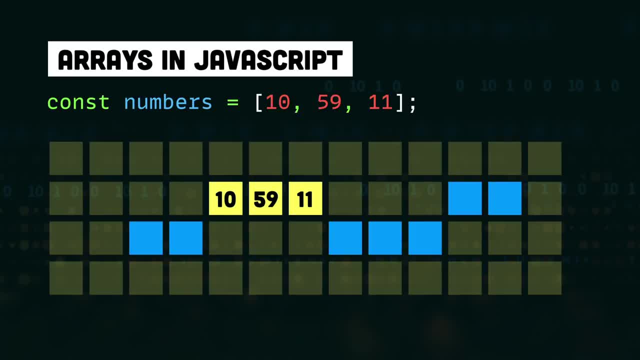 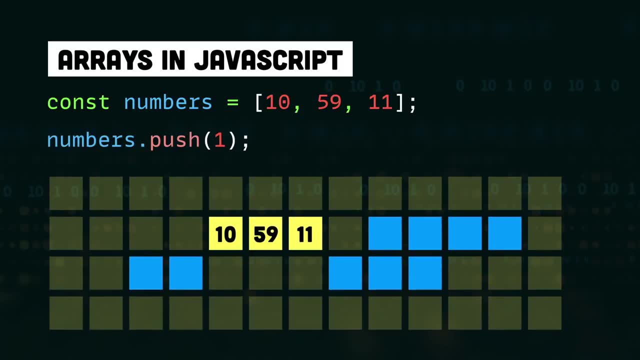 And our program is going to continue and keep using the other blocks in the memory for other stuff. Later on, when we push a new number to the array, it's going to check and see if the next block is empty for us to consume or not. If it is empty, it will allocate that for our 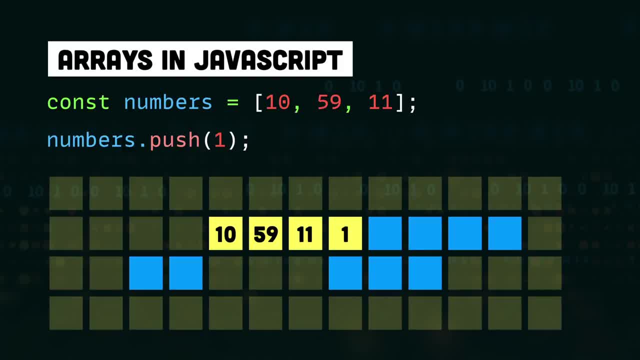 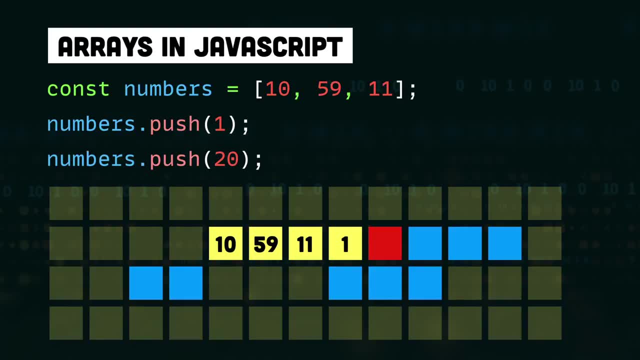 array and put a newly added number to that block. and now if we try to push a new number to that and let's say that the next memory block it can't be allocated, in that case it is going to try and find out some other place in the memory where it. 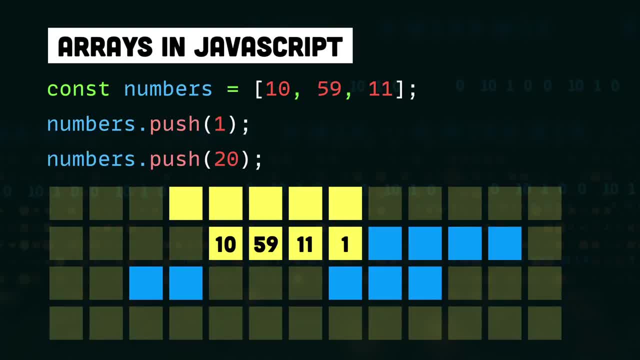 can populate the whole array. it is going to find that space, allocate that for the array that we have, move all the items that we have in the array there and free up the previously allocated array space and push the new item to the newly allocated array space. and that is how these languages can. 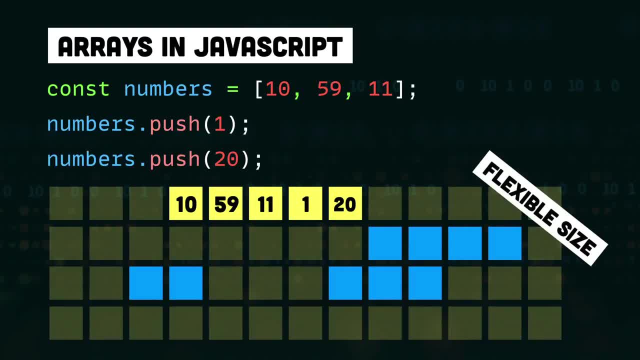 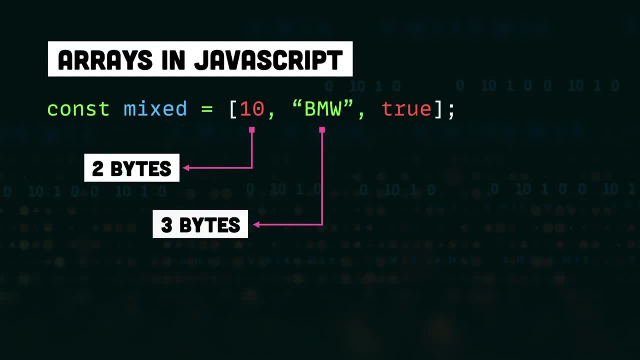 have dynamically sized arrays. now the next question is about the arrays with the mixed type values. here we have an array with an integer of two bytes, string of three bytes and a boolean of one byte. how is javascript able to represent this array with the mixed type values and the 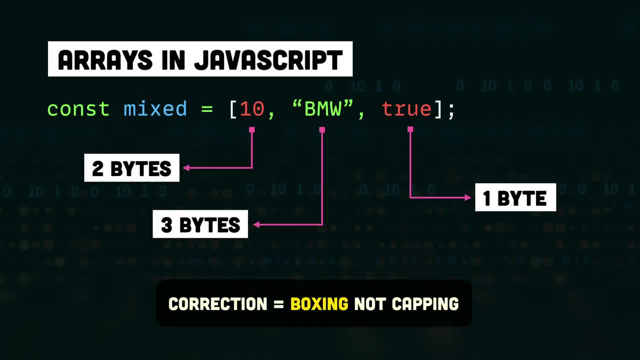 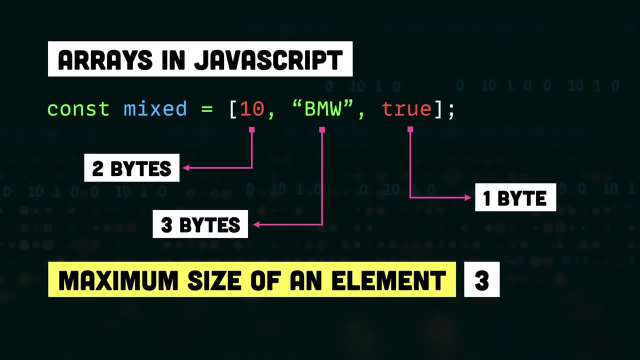 answer to that is the capping of the size. so what do we mean by that? now, in this case, javascript is going to find the element with the maximum size in the array. now, in this case, string is taking the maximum size of the array and it is going to find the element with the maximum size of the 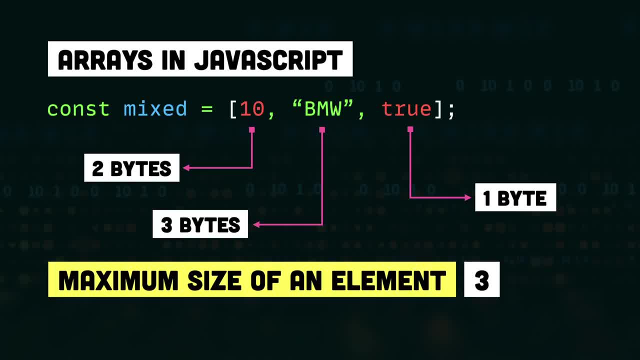 three bytes. so it is going to take three bytes and allocate them for each of the element of the array. so in total it will allocate nine bytes- three bytes per element in total for the whole array. so instead of seven bytes we'll have nine bytes for this whole array. let's look at the visual. 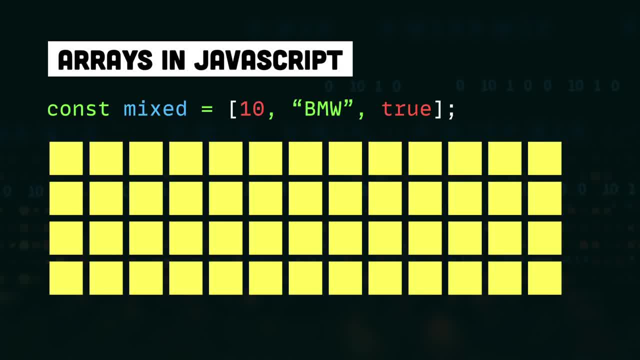 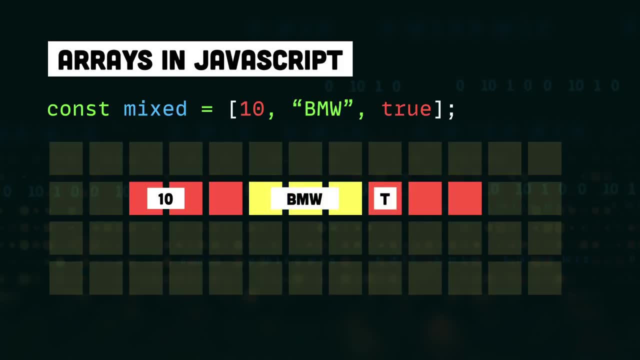 representation to understand more. so first we have the integer instead of allocating two bytes, since the maximum size of element in the array is three bytes. so it is going to allocate three bytes for the integer, then three bytes for the string and three bytes for the boolean. now, when it comes the time to read the values from the memory, it knows that 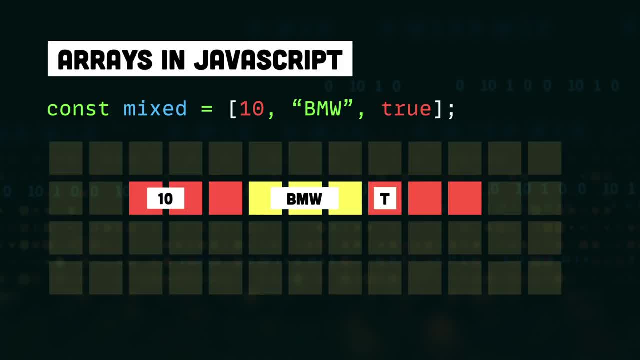 it has capped all the elements to three bytes. so it is going to read three bytes and get the first element, skip three bytes, and read the next three bytes to get the second element, skip six bytes, and read the next three bytes to get the third element, and so on. and that is how it. 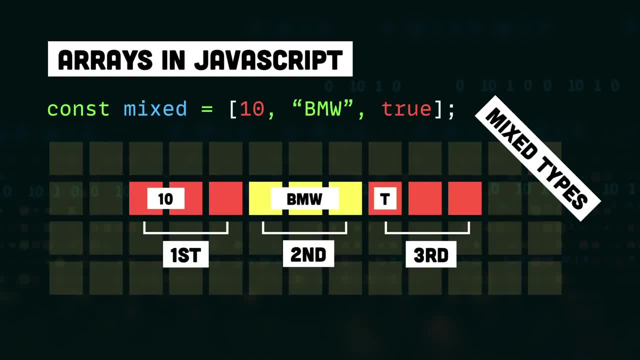 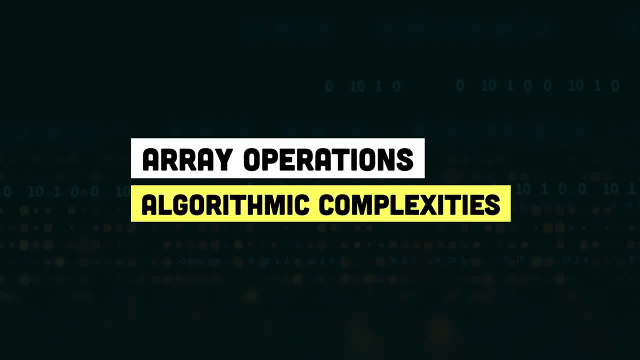 gives the possibility of elements having the mixed types in the array. all right, so now that we know what the arrays are and how they work, let's look at the operations that we can perform on the arrays and the algorithmic complexity of those operations. let's say that we have this array. 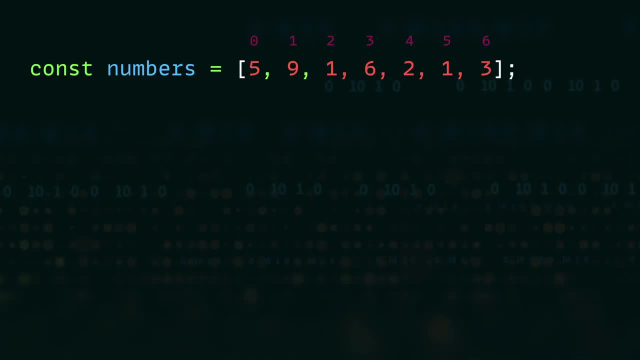 of numbers, the items of the arrays are indexed, starting from zero till the end, and we use this index to read the elements from the array. so, for example, to read the first element of the array, we will write numbers of zero and we will get the first element of the array and we will get the 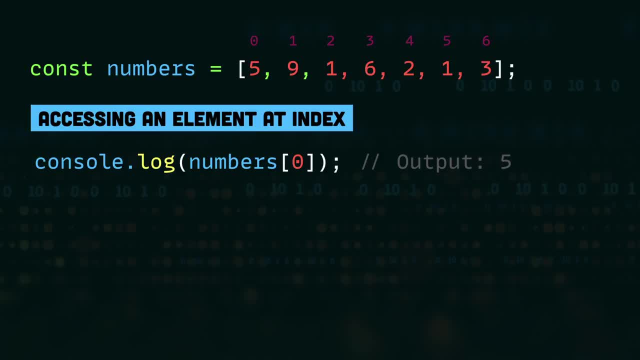 first number and to read the fifth element of the array, we will write numbers of five and so on, and the complexity of reading an element from the array is constant complexity, that is o of one. we will not be discussing how the complexity is calculated in this video, but i have a separate